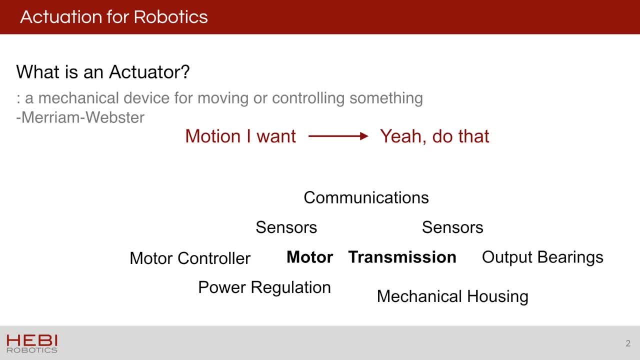 power it. You need to be able to communicate between all these sensors. There's mechanical considerations in terms of how actuators you know physically fit into your robot, And I'm not going to talk about it here. but there's a whole other side in terms of 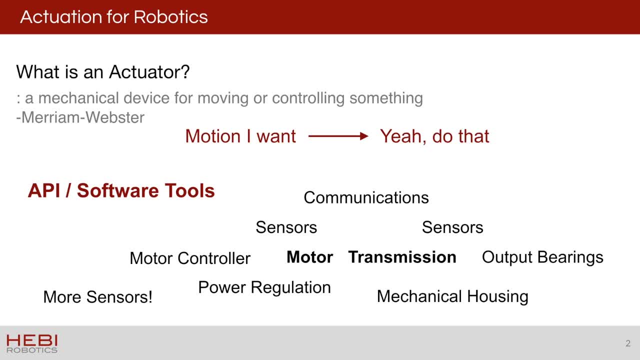 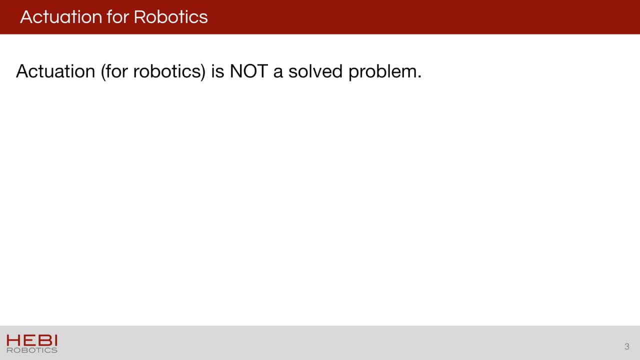 the software tools we use and provide to control actuators that are really just as important as the physical device. So why are we even giving a presentation on this? I would contend that actuation for robotics- the kinds of people that are watching this presentation- it's not a solved problem, right? Electric motors have been 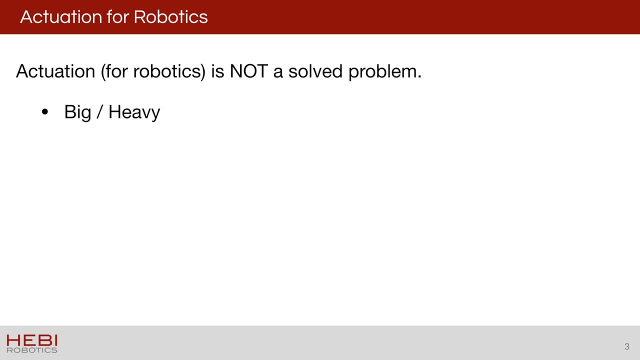 around for, let's say, you know, widely available for like 100 years. Gears right Transmissions have been around for even longer than that, But they're still. the widely available ones are big and heavy for what we want to do. right, We're trying to create systems that are on par or 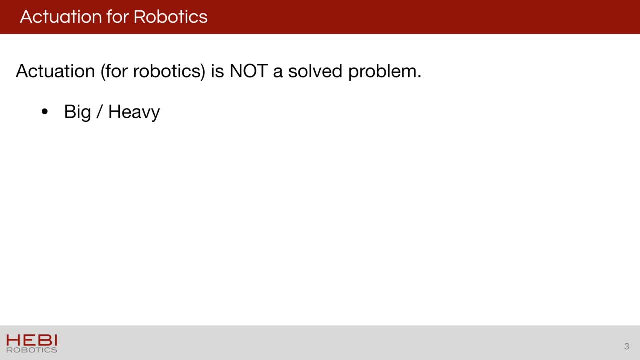 exceeding the standard. So we're trying to create systems that are on par or exceeding the standard. So we're trying to create systems that are on par or exceed or closely interact with humans, and that's still not broadly available. Industrial robotics has made huge strides over the last. 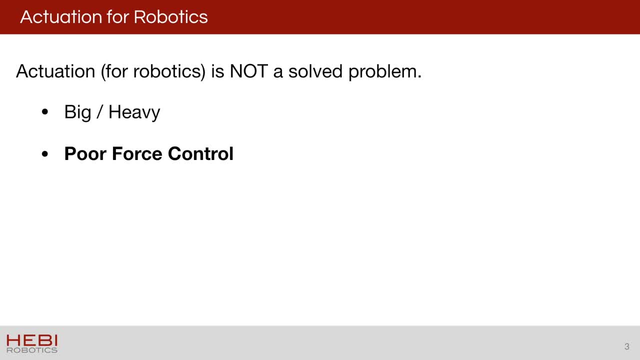 let's say, 30, 40 years. but it's done it by really focusing on position control and being, you know, rigid, precise kind of superhuman in that ability. But things that people are exploring now really focus on force. That's not really broadly available If you try to solve. these kind of power density and force control problems. you're going to end up with a lot of things that you're not going to be able to do in the future. You're going to end up with a lot of things that you're not going to be able to do in the future. You're going to end up with a lot of. 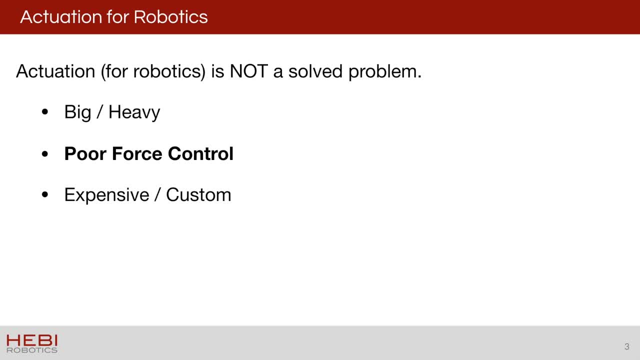 things that you're not going to be able to do in the future, You're going to end up with a lot of control problems. You wind up with something that's frequently expensive and custom. It's also complicated to control and the things that you need to solve aren't exactly the things that 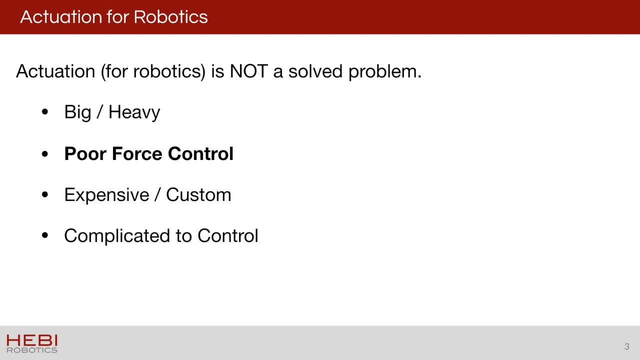 are taught broadly in kind of high school or undergraduate robotics courses, And we all in this field suffer from the fact that it's pretty niche right. It's low scale, There's not a lot of standardization, So a lot of groups wind up rolling their own in this area, So it's very 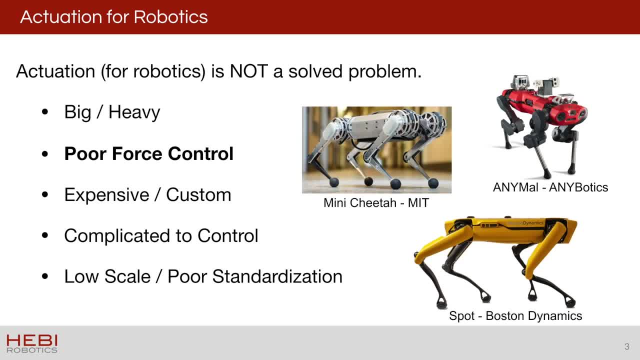 fragmented. It's not a perfect example, but three groups out there today that make quadruped robots have all chosen to make their own actuators And I think for pretty good reason. Their use cases all differ subtly. Their scales are slightly different in these sorts of robots, But really it's a niche. 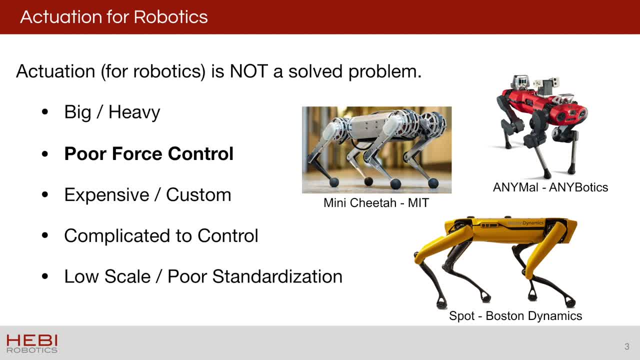 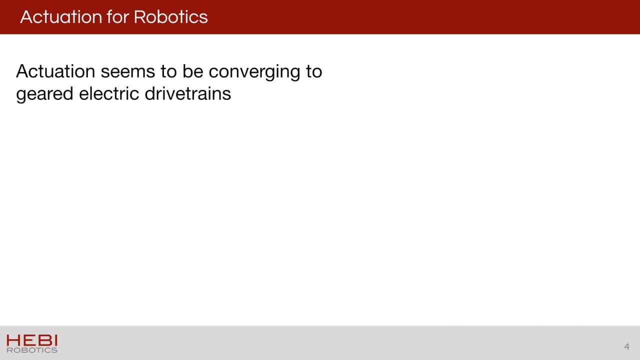 field, and the tools that these people need to accomplish their jobs just don't exist, So they wind up rolling their own actuators from the ground up. So if you do have to make your own actuator or you're choosing among actuators, I think the trend does. 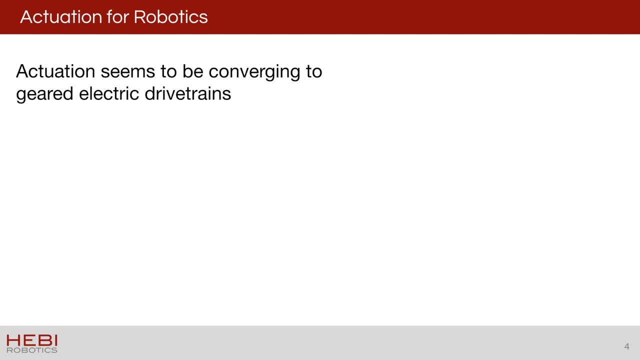 seem to be, finally, that things are really converging to geared electric drive trains. So taking an electric motor, usually a brushless electric motor, putting a mechanical gear train on it and using that as kind of the core motive part of your robot. So if we follow- it's not a perfect example, but if 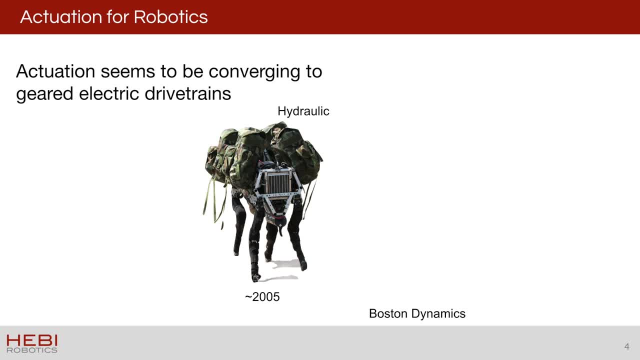 we follow a robot, it's not a perfect example. but if we follow a robot, it's not a perfect example. So here's a picture of Boston Dynamics from when they first came really onto the scene publicly with a robot called Big Dog in the mid-2000s. That was a hydraulic robot that was powered by a gas. 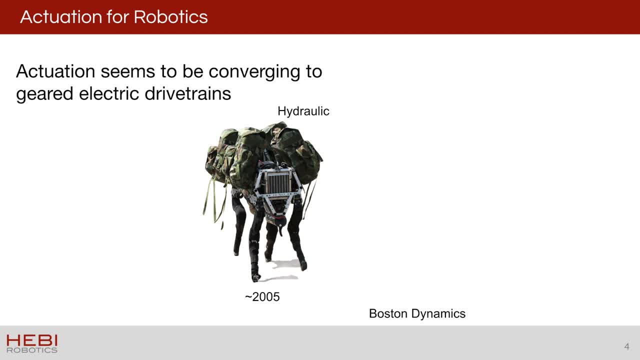 motor and a hydraulic pump to drive hydraulic actuators in the legs. Ten years later they had progressed to an electro-hydraulic robot called Spot, where there was now electric motors driving still hydraulic actuators in the legs, and you can see that they've been using that robot for a 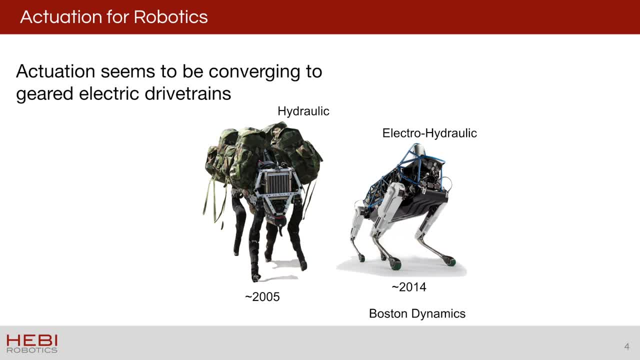 you could see the improvements in control that were able, uh, that they were able- to do because of that, Uh, and today, though the spot that they're selling today is electric motors and gears, Hydraulics is is out of the equation, Um, and this isn't a perfect example, right Like? 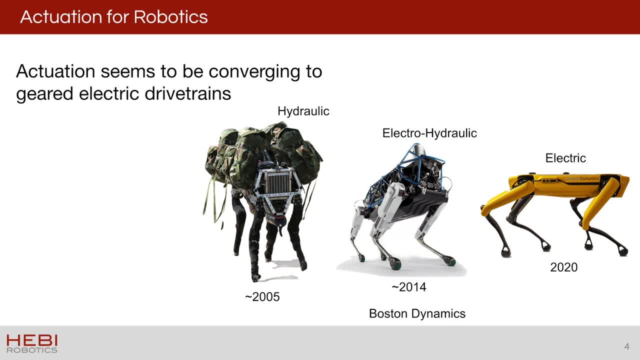 there's been changes in scale going down, but I think uh, electric motors have kind of risen up to meet the challenge as well, uh, and kind of met them halfway. So we've there's been improvements in understanding how to make and especially control electric motors, uh, and especially 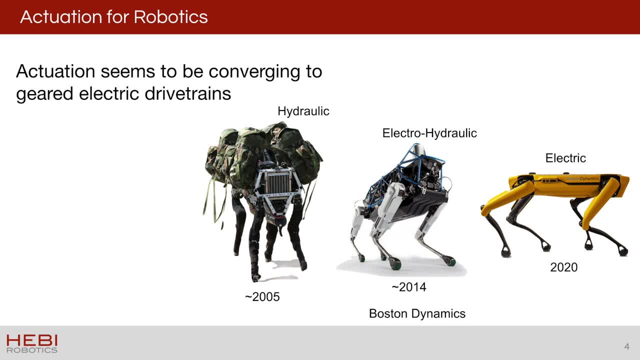 controlling the peak performance of electric motors, and that's continuing to improve. So, the same wave that Boston Dynamics is riding, I think the rest of the industry is riding too. Uh, there are other options. Uh, I think I think of these that I'm going to list out really mostly as 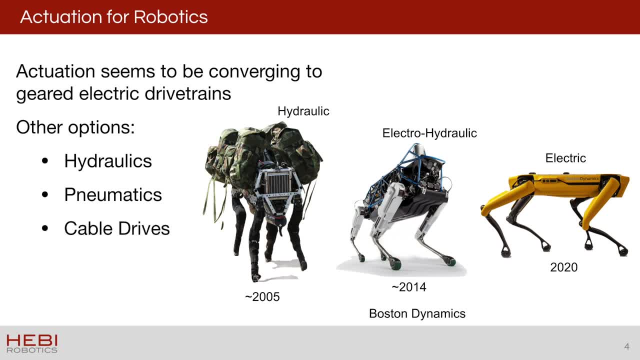 transmissions, So hydraulics, pneumatics, cable drives, and then you know, lastly, direct drive. no, no transmission. All of these things that I'm listing kind of, I think, used to be, in a sense, discrete forms of. 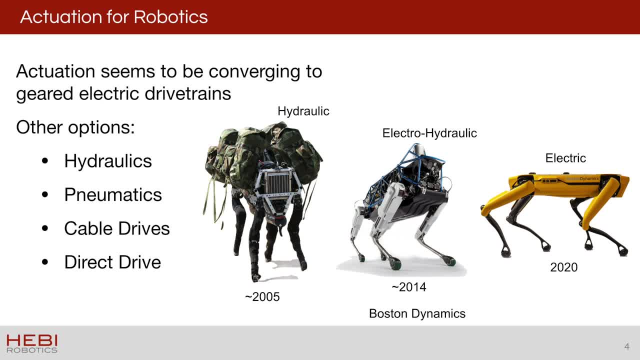 actuation. but now I really think of these, uh, in all cases, are probably going to be driven at some point by an electric motor. Uh, and there I really think of them more as as transmissions rather than actuation technologies in and of themselves. Um, so why are electric motors? 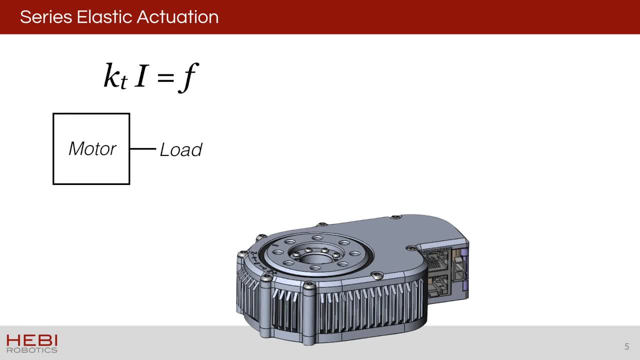 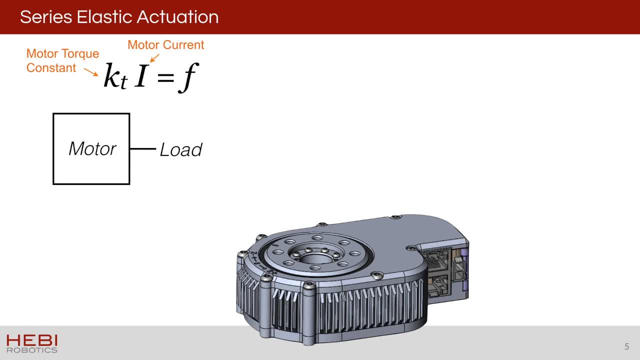 constant, uh, which is, uh, basically a set property of the motor, Uh, and if you multiply it by the motor current, which we can usually measure pretty good, you have the force, the, the torque that the motor's putting out. Now the downside is: is, in reality, you usually have a. 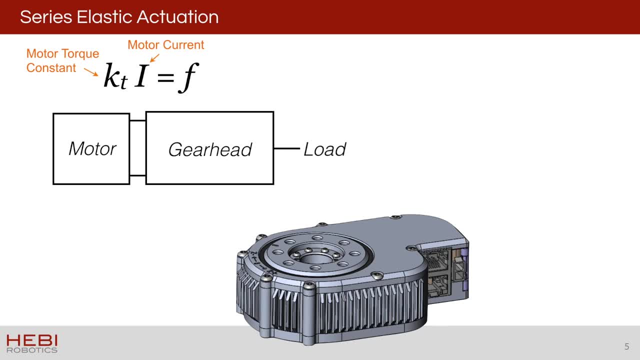 gear head, uh, between your motor and the load that you're trying to control, And with a lot of gear heads, that basically breaks this relationship. So, uh, there's a lot of there's a lot of relationship. You can no longer use motor current to determine your force. Uh, one workaround to. 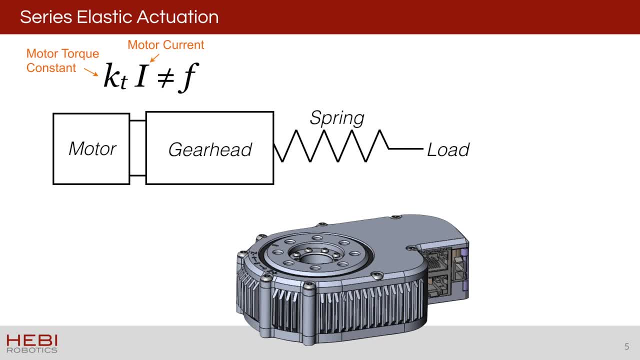 this problem, which uh Heavy Robotics uh has a lot of experience with, is to put a spring on your output, And this is called a series elastic actuator, because you're putting an elastic uh member in series with the rest of your actuator And what this does is this turns. 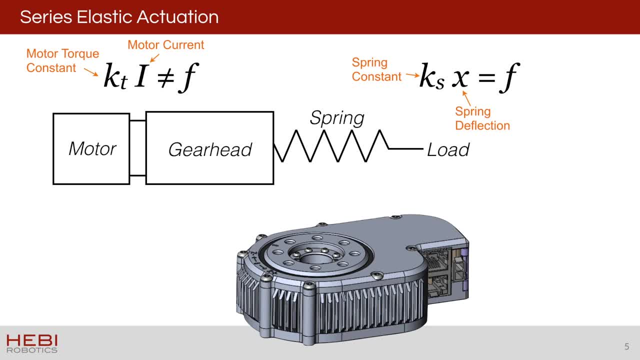 your force control problem, because sensing force is hard- into a uh position control problem, uh, which is uh a lot easier. right, The same encoders we use to measure position. If your deflections of your spring are now large enough to measure as a 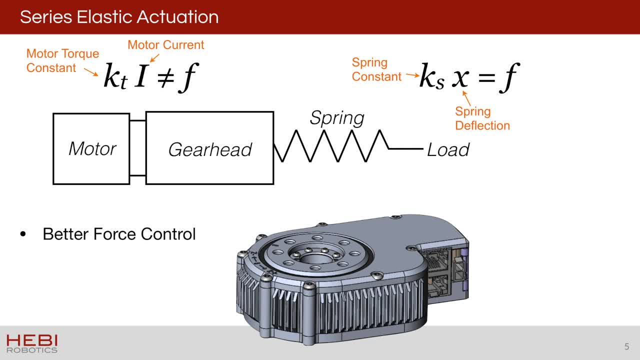 position. you can do that as well. And uh series elastic actuators have the benefit that, because we're essentially low, passing the output, uh, we have better force control. Forces evolve more slowly, We can control them more stably. Um, but that same trade-off means. 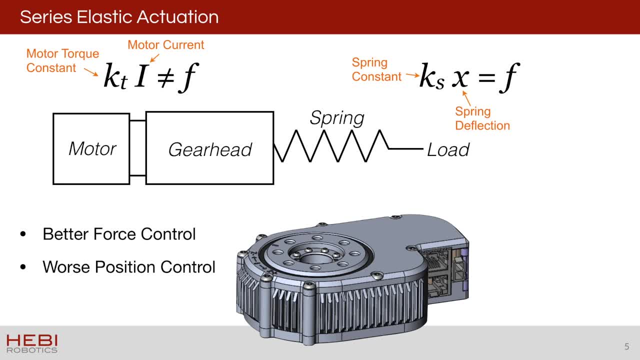 that we have worse position control, We're less stiff, We're not as rigid, Um, so we kind of lose out on that superhuman, uh position control performance that you get out of industrial robots. And then one last that I'll put as a benefit is: uh, you get shock. 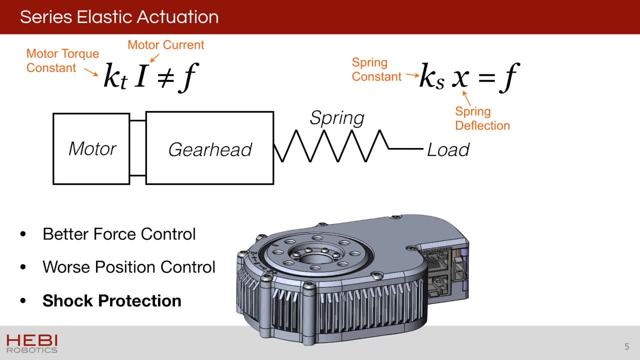 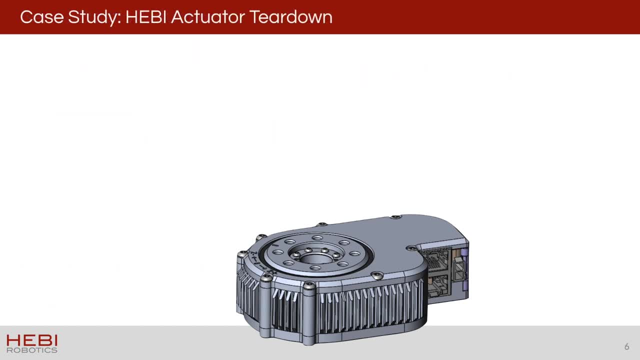 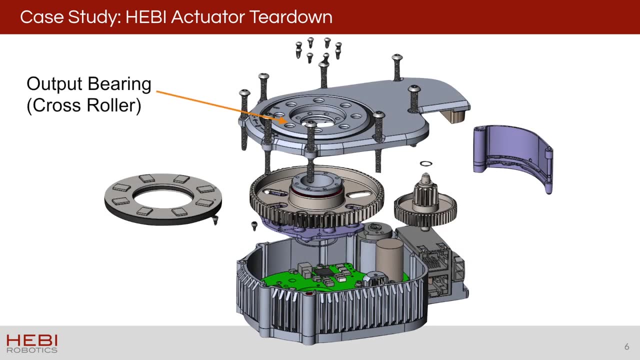 protection. right, Your, your, uh. compliance on the output protects a lot of the inside of the actuator, much, much like the suspension of a car protects the frame of a car. So to make things more concrete, let's do a kind of a breakdown of Heavy's X-Series actuator Working from the 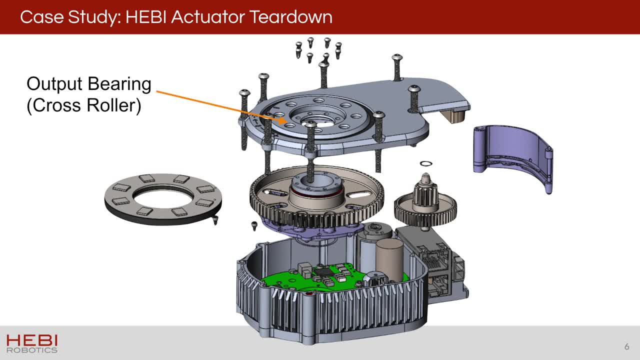 output bearing, which is really one of the most important parts of an actuator, right, It isolates whatever you're doing to the outside of the actuator, to whatever's going on on the inside, Uh. so in this case we use crossed roller bearings, uh, which provide not just radial 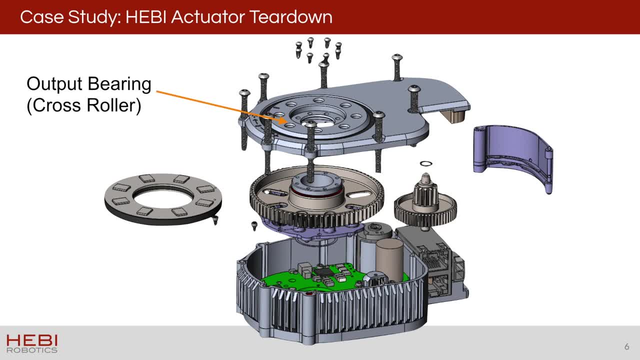 and thrust load, but especially cross moment load. So if you're essentially springboarding something off the actuator, like if it's the base of an arm or a base of a leg, um the the case of the, the actuator bears all the load, which is super important. Uh, we have a spring on. 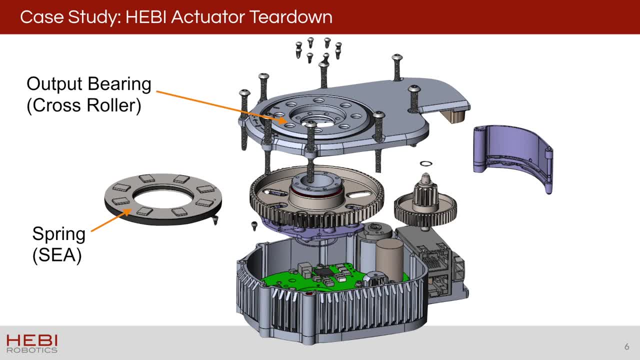 the inside of the actuator. We have a spring on the inside of the actuator. We have a spring on the inside which is kind of a level of complexity that a lot of other actuators uh don't if they're not series elastic. Uh, we have output encoders to sense the deflection of the spring. 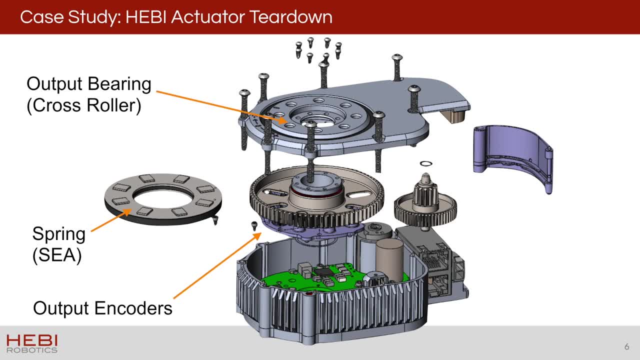 but also we believe in sensing the output of the actuator directly, kind of with as much precision as you can. Uh, that has advantages, even if you do mostly care about force. Uh, we have electronics inside the actuator that are really tightly integrated with the unit for 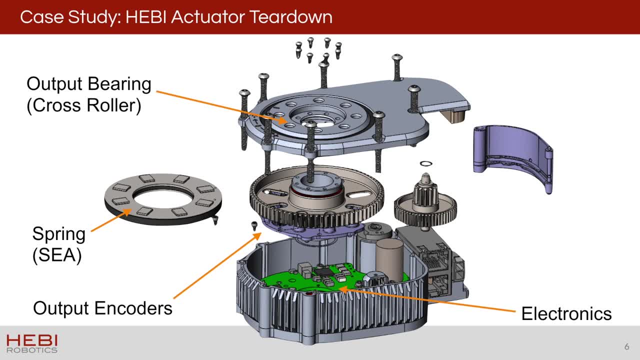 size, Uh, we try to keep everything down to a single circuit board, Uh, and we have spur gears right Part of our transmission, Uh, and we try to reuse components wherever possible, uh, really, to achieve scale, You know. lastly, we have that motor, We use the 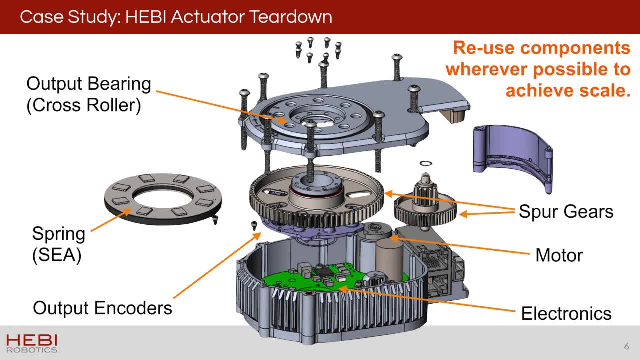 really two variants of a motor across all of our actuators. We use the same electronics across all of our actuators, the same output bearings across all of our actuators. Um, again, because we are in a low scale sort of niche environment, it's really important to be able to up quantities. 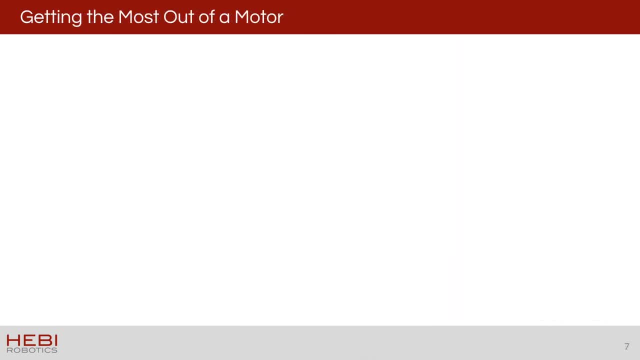 wherever possible. So, uh, we have a lot of components that are really tight, but we have to try to drive down price because we don't have the benefits of really large markets like, uh, automobiles or cell phones, In terms of getting the most out of that motor that we 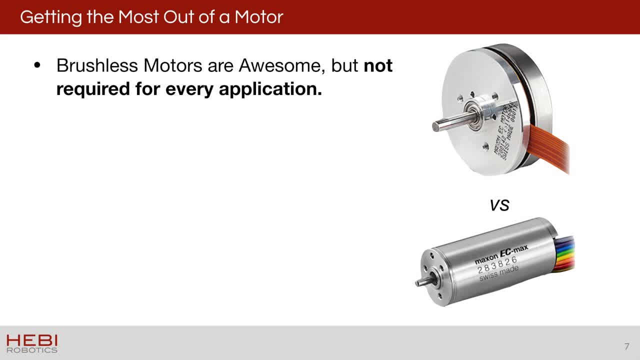 choose to put in the actuator. um, brushless motors really are kind of you know the way to go. They're dominating the market, but I will say that, uh, they are not required for every application. They do have drawbacks in that, um, at certain scales they are expensive. 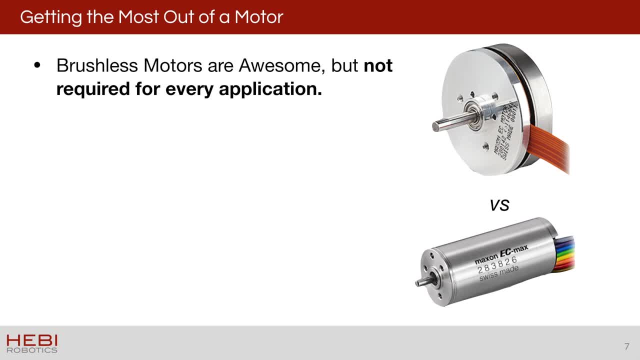 Uh, they are also difficult to control really at at low speeds. Um, so there are certain things where, if you're not really space constrained, power constrained, power density constrained, uh, old brushed DC motors can have, still have a lot of advantages. So don't feel like your. 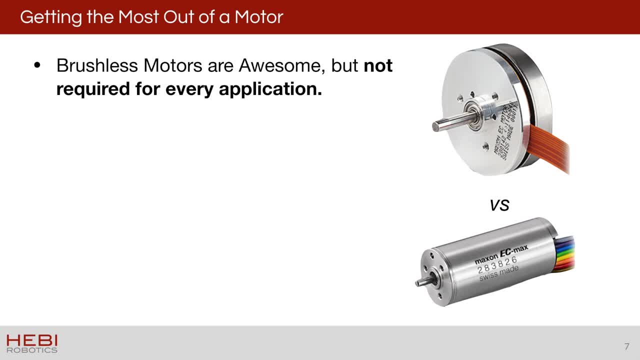 application requires a brushless motor out of the gate. if you're designing your own actuator from scratch, Uh, I will say that you do have to think of a motor, really in conjunction with its transmission, right Like so, if you know you need a harmonic drive, for you know a motor that's 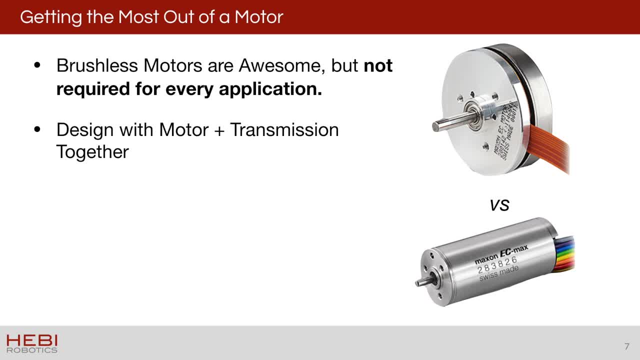 torque density or especially for lifetime reasons. essentially, a lot of your choices in motor have already been made for you. Um, and so you're, you're going to look at more of a large gap radius motor. Uh, one thing I'll say is I think of speed now as kind of a, a soft constraint in a sense. 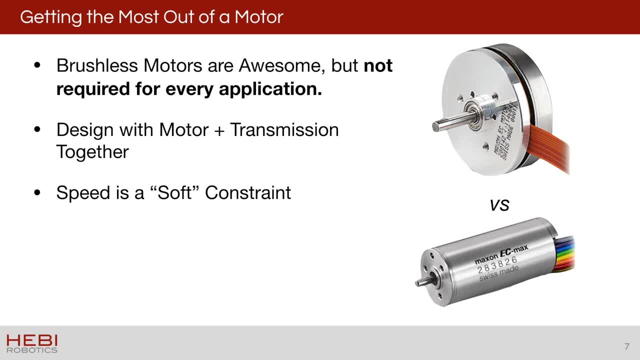 that, given enough voltage, you can really run most motors as fast as you want. Um, and what the bearings? and in a lot of research systems that's okay, right, Um, bearings are often rated for tens of thousands of hours of lifetime And a lot of research systems live in the hundreds of 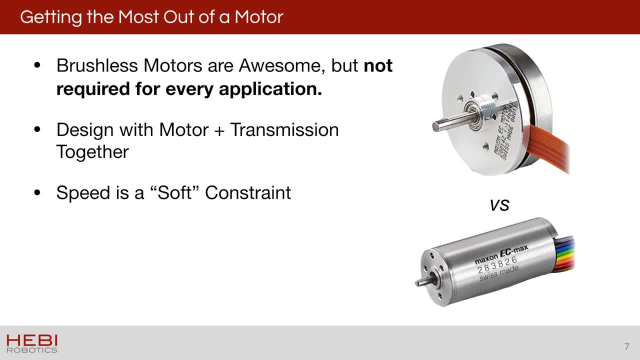 hours of lifetime. So if you're kind of making, trying to make a trade-off between torque and speed on your components, um, if you have a uh, if you have knowledge of really the lifetime, you can really treat speed as a soft constraint, Whereas uh, torque, if you exceeded you can. 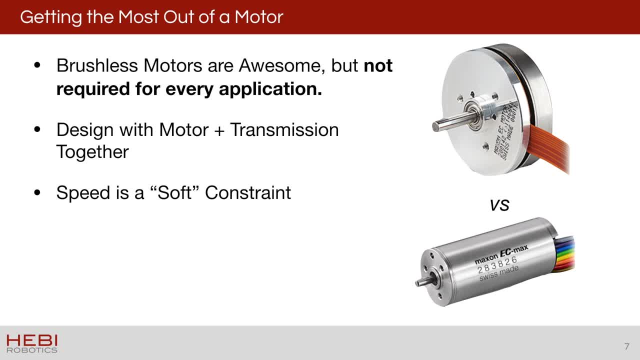 mechanically damage or permanently damage your, your motor. So, uh, if you're, if you're, if you're either thermally or mechanically so, torque is a hard constraint And really most of the gains to be made, uh, in terms of pushing the envelope, are really based on the thermal characteristics of 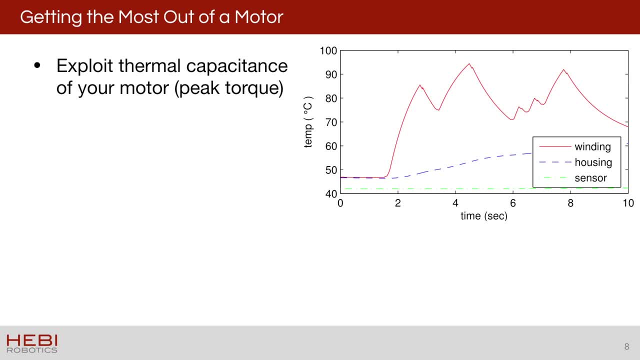 the motor. Uh, so at Hebi, we you know we believe a lot in exploiting the thermal capacitance of your motor, right? So how much? how much heat can your motor temporarily absorb, based on what you're trying to do? Uh, and it's worth putting a fair amount of work into understanding the true winding. 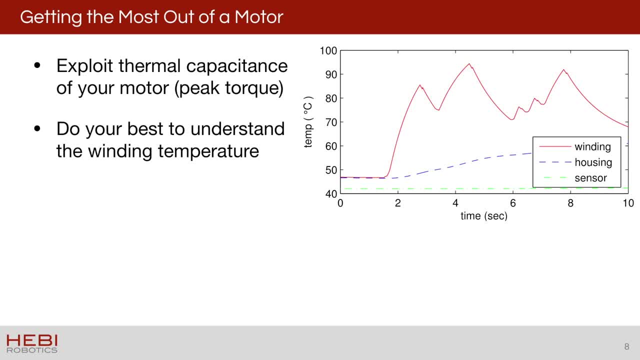 temperature of that motor. Uh, very rarely can you actually get a sensor into the windings of a motor. So, uh, really, make use of tricks to give yourself a sensor and it's okay to even think of it as a sensor. Uh, if, um, even, 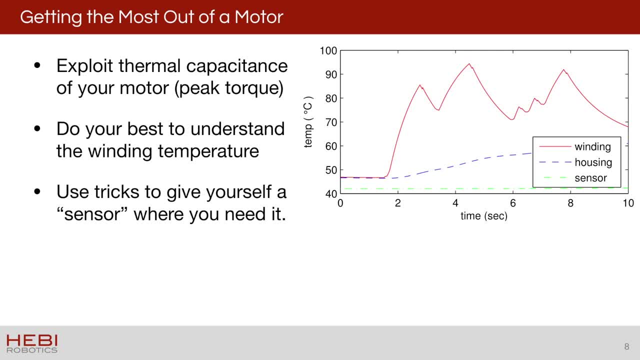 if it's really just derived from uh a bunch of other things. So, for instance, in our actuators, we do not have a temperature sensor in our windings, but we have a temperature sensor next to the case of the motor, which is what this green line is in this plot from uh. 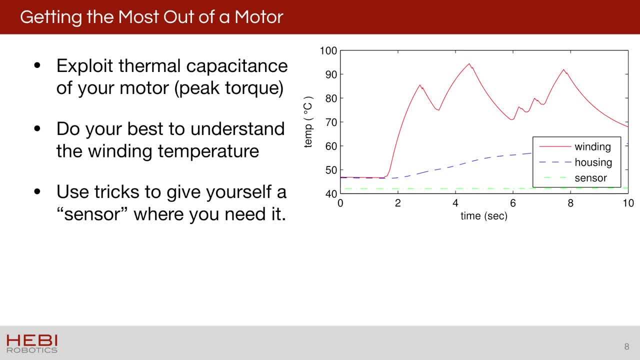 from our actuators. But we also know the speed of the motor very accurately, We know the voltage going to the motor very accurately, We know the current going in the motor very accurately, Uh, and we can use all of this plus uh information from the data sheet, plus uh things that we've done to verify. 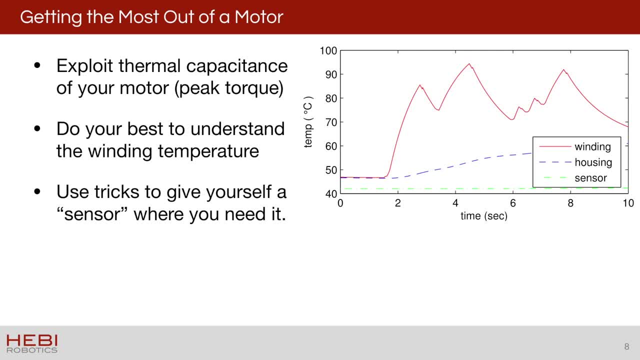 and testing, uh, to verify what and estimate what the uh, what the temperature of the windings really are. And lastly, I'll say a little bit of, a little bit of cooling goes a long way in motors, Again, thermal, thermal limits really are. 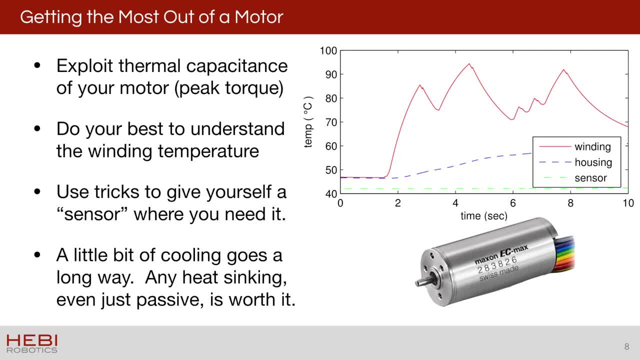 The, the, the thing that holds motors back. So wrapping your motor in a little bit of metal or blowing the slightest breeze you can, um does a lot to to get performance. So in our case, just wrapping, wrapping our motors in in a two millimeters of aluminum and sinking that to the 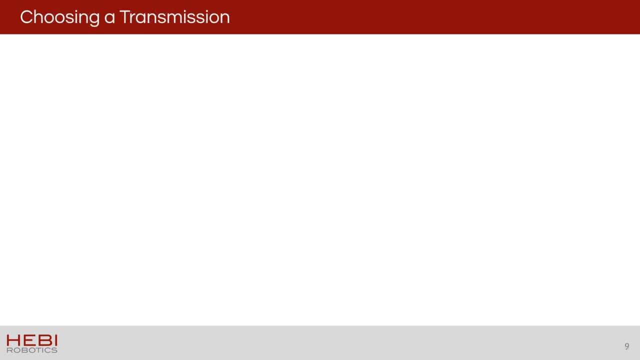 case uh essentially doubles the performance of the motor over it sitting in air In terms of choosing a transmission. um, this is kind of my personal opinion, um which I don't think it's aone that I would be too uh to be too hung up on on kind of data sheet. 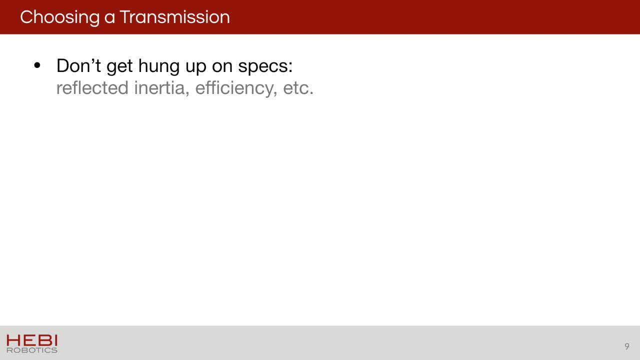 specs, A lot of people think, oh, I really need to minimize reflected inertia, or it should really focus on efficiency, And in my experience, a lot of these things kind of come out in the wash right. So if you're, if you have a wide variety of gear, trains, and you're focusing on reflected 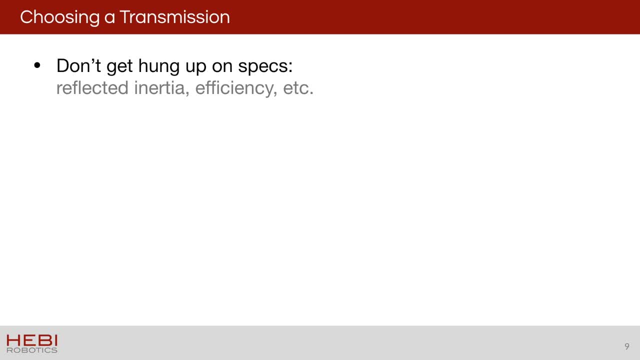 inertia. well, the kind of motor that you're going to use on a 12 to one gear train has a lot more inertia than a motor that you might be using on a thousand to one gear train, coming out to be roughly equivalent. Uh, and also in terms of efficiency, right, Efficiency. 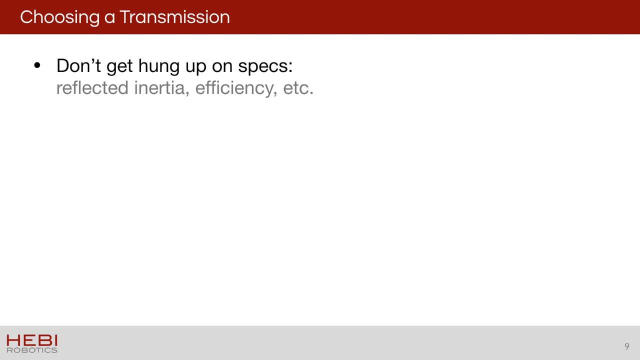 for a motor is frequently defined at, uh, a very high, a reasonably high torque, at a very high speed. A lot of robots spend a lot of time at stall, So maybe really I squared R? um, you know, uh, uh, jewel heating is is what you're really should be focusing on, Um, so don't get hung up. 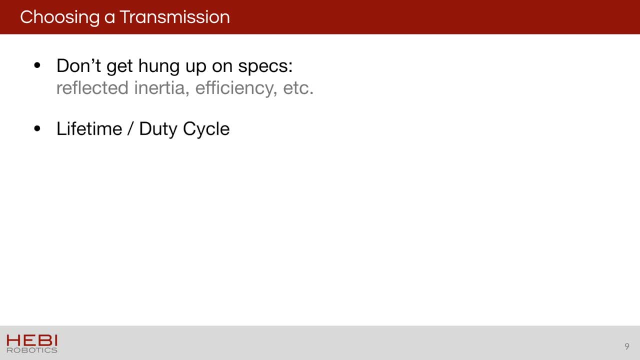 on kind of traditional specs. It's much more important to focus on the expected lifetime of your actuator. Is this an industrial application where it's going to run for 10,000 hours, Or is this more of like a formula one robotics competition thing where I can really push the? 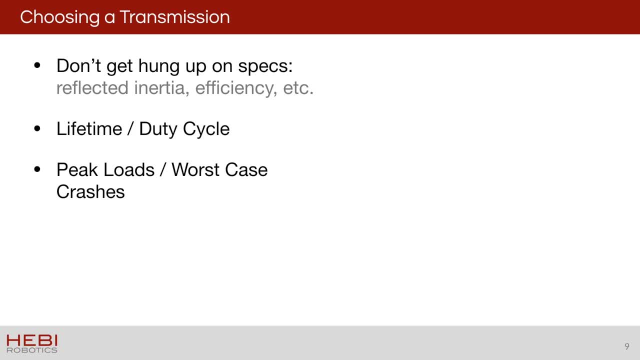 envelope, Um, understand what peak loads of your robot look like and understand what the worst cases are. So like. if you're making a robot that can fall down or bang into things, give some thought as to what that looks like. uh, you know, kind of mechanically through your actuator And 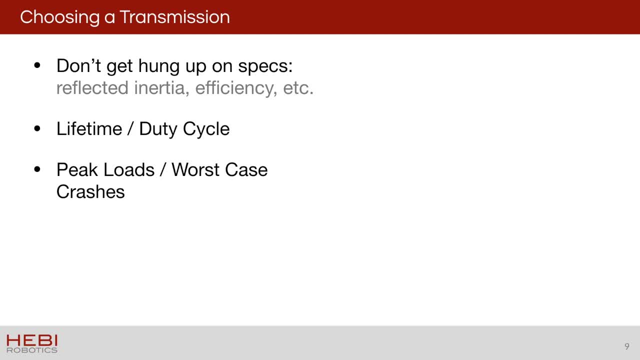 that might drive um very different choices in terms of transmissions or things like series elasticity. Really, really, as much as possible. give a thought to how many man hours it takes to maintain a system, or what I kind of call fiddliness right, How repeatable is it? If do I, if I need to make one of something? 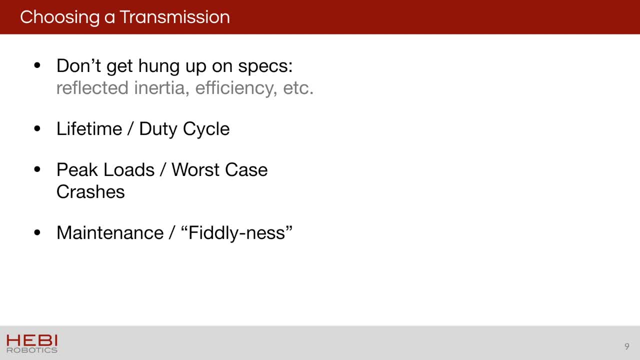 it's okay if it's a little fiddly. Uh, if I need to make a hundred of something, it needs to start to be a lot more manufacturable. Um, and this is something where where cable things, like cable drives, start off looking very appealing and then the the maintenance aspects of them, uh, become a 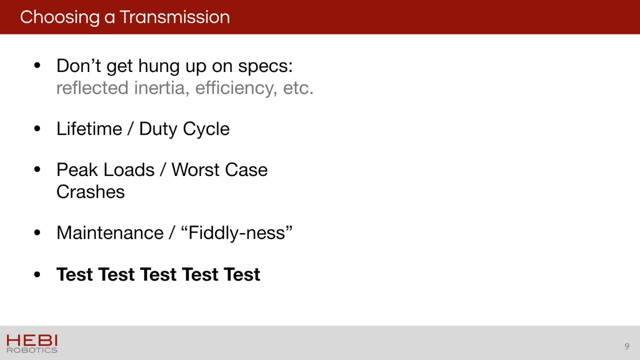 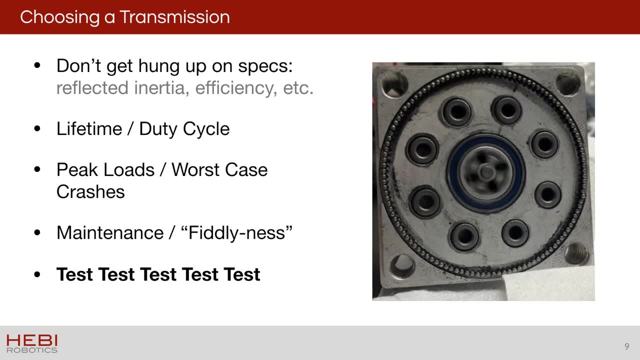 big, big drawback. And lastly, I'll say: test, test, test, test, test, test, test your thing as much as you can early on. Um, an example of this that I'll share is: uh, uh heavy. uh spent a lot of time.